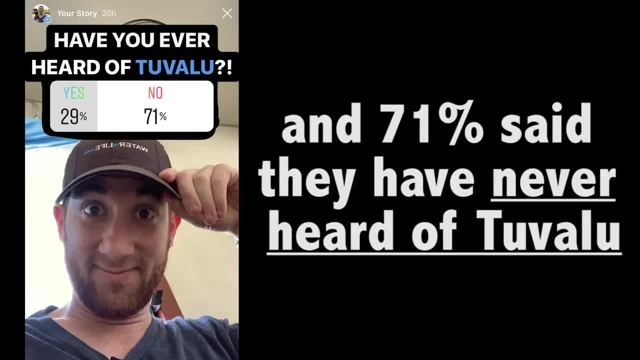 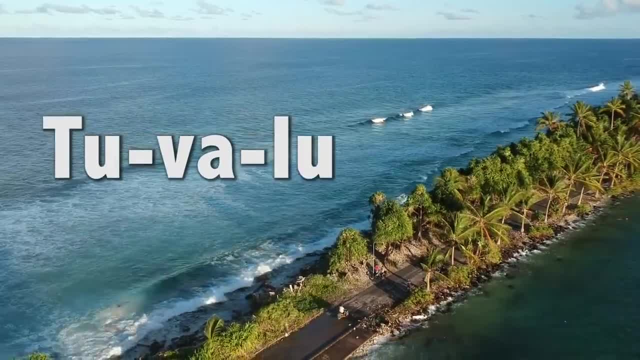 and 71% said they had never heard of Tuvalu. That's pretty absurd, considering that they're a real sovereign country with voting power in the UN. Tuvalu, Tu-va-lu- The name itself makes me curious. Wait, so Tu-valu? 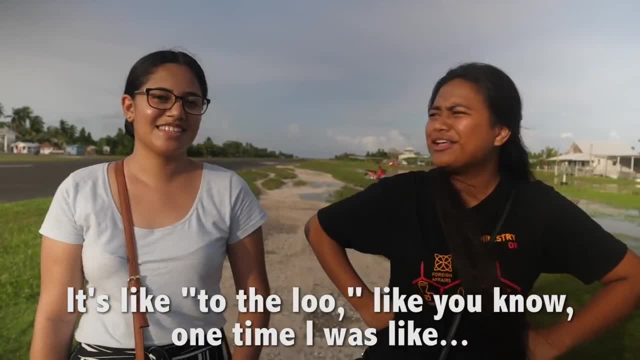 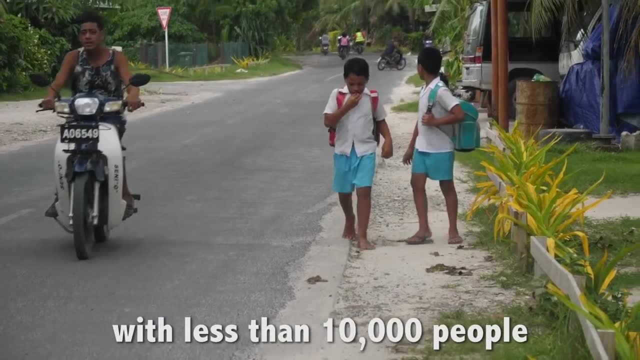 Tu-va-lu, but an American would say Tuvalu. It's like to the loo. like you know, one time I was like dude. that sounds like to the loo. It's the world's four smallest country, with less than 10,000 people. 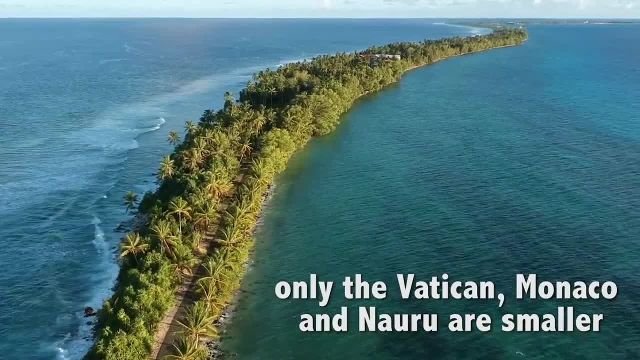 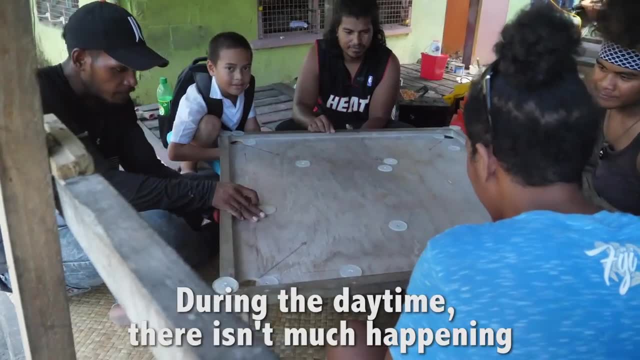 Just pretty much chill. Only the Vatican, Monaco and Nauru are smaller. This is the only prison here in Tuvalu. The front gate is not even closed During the daytime. there isn't much happening. I'm walking down the main road here and there is nobody around. 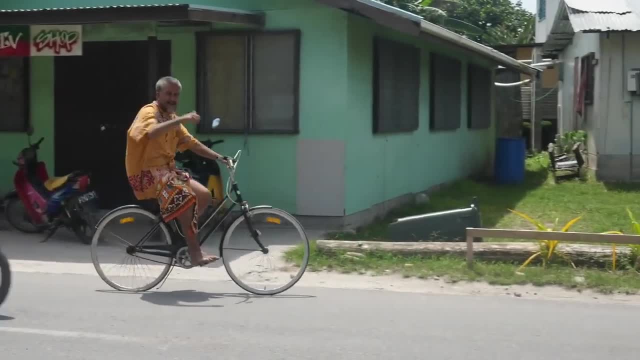 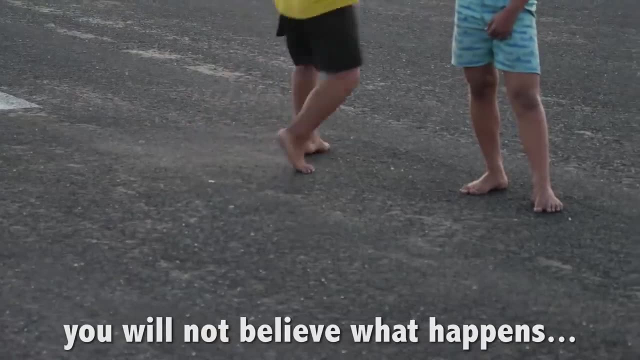 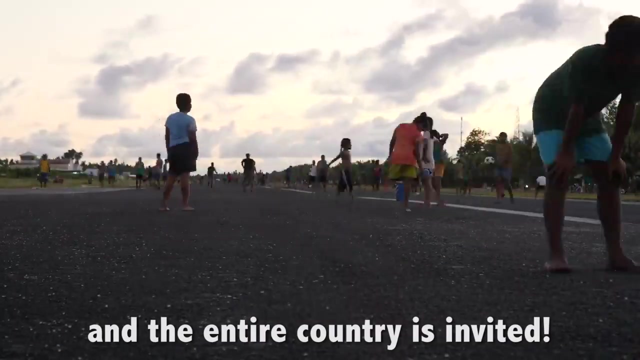 And it's always really hot, But around 5pm every evening, as the sun starts to set, you will not believe what happens. The airport runway turns into a massive playground And the entire country is invited: Soccer, volleyball, basketball, rugby, running and even their own invented sport. 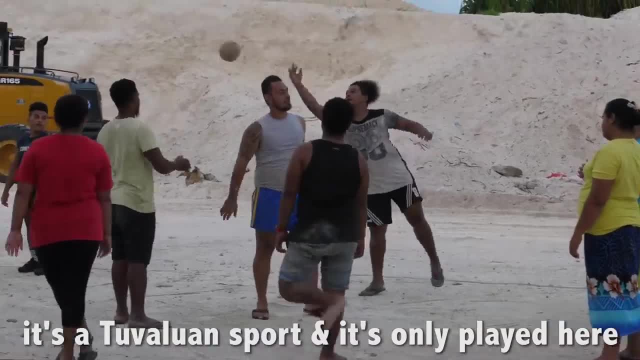 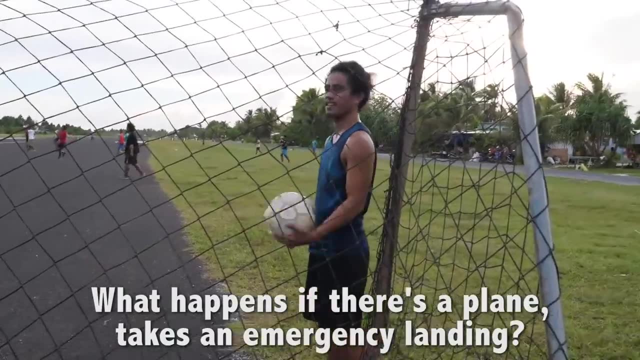 This sport is called Te Ano. It's a Tuvalu sport and it's only played here. Do you play here every day? Yeah, every day. Oh yeah, Every night, Yes. What happens if a plane takes an emergency landing? 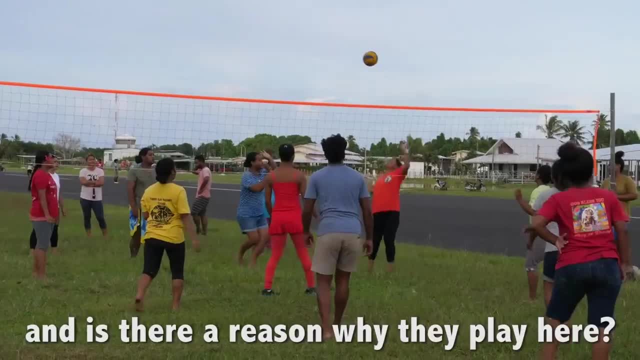 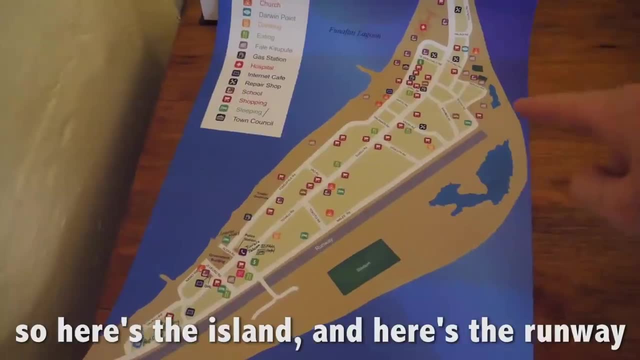 What happens? Oh, usually they'll have a siren for it, And is there a reason why they play here? I think it's because it's the only big, large space that we have on the island. So here's the island and here's the runway. 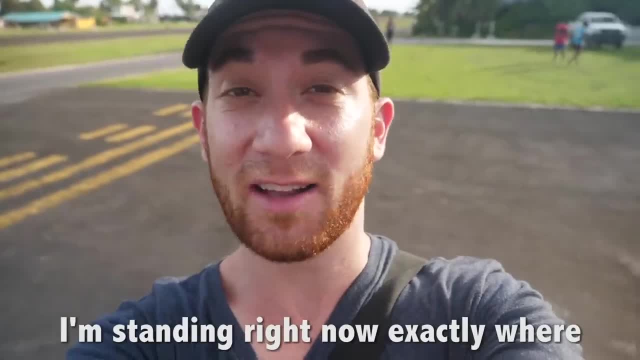 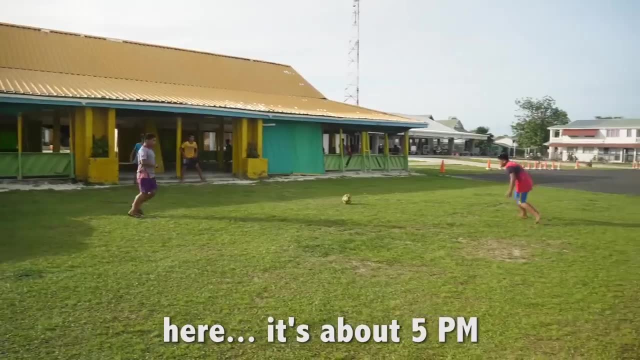 It takes up the entire length. I'm standing right now exactly where our plane arrived just a few hours ago. If you remember, I showed all the people waiting in this little building And now all the kids are playing soccer here. It's about 5pm. 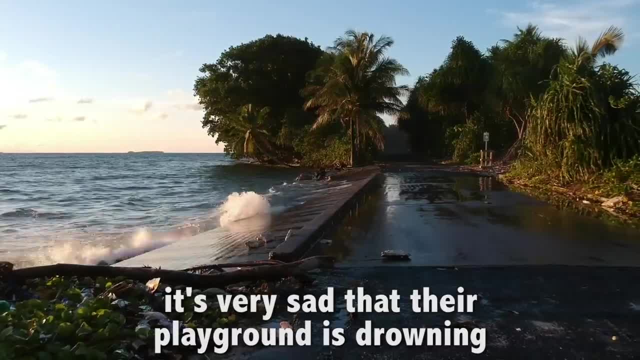 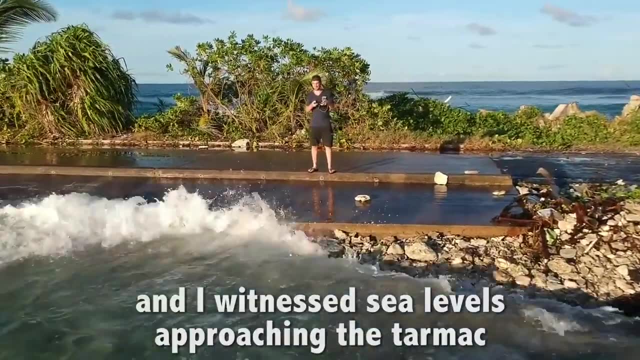 While this is one of the happiest environments I've ever seen, it's very sad that their playground is drowning. I just happened to visit Tuvalu during the highest king tide ever recorded And I witnessed sea levels approaching the tarmac. It just keeps on creeping, creeping closer. 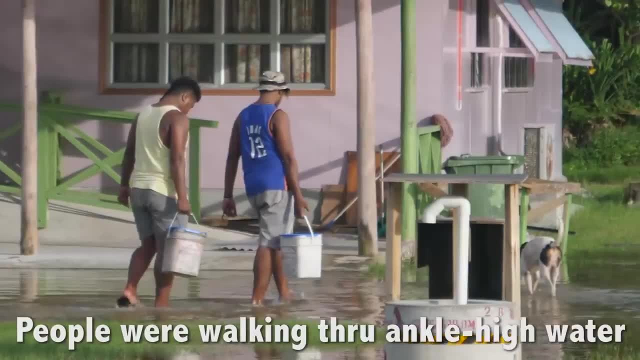 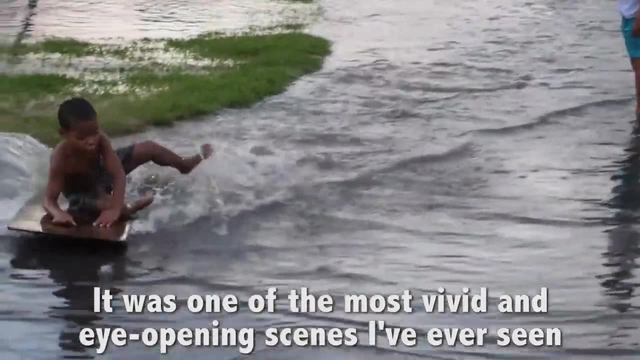 Soccer games turned into water sports and splashing contests. People were walking through ankle-high water just to cross the airport. It was one of the most vivid and eye-opening scenes I've ever seen. The kids have no idea that they're playing in the ocean.